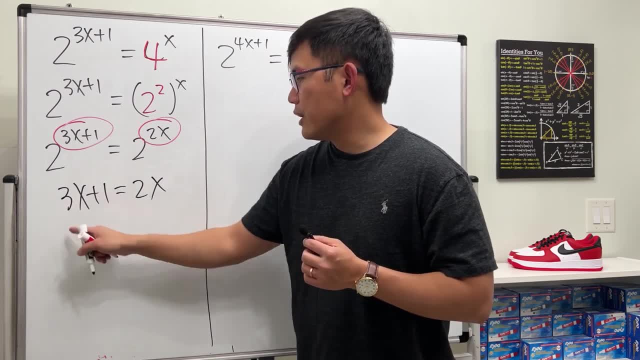 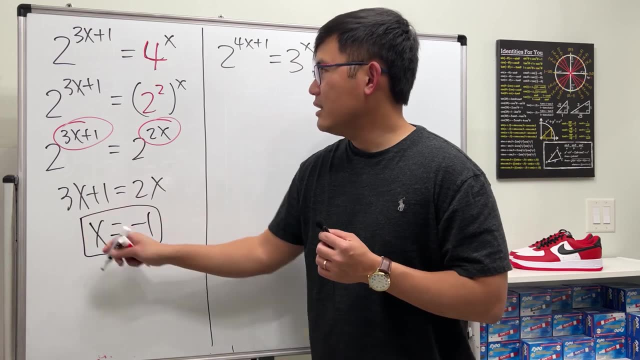 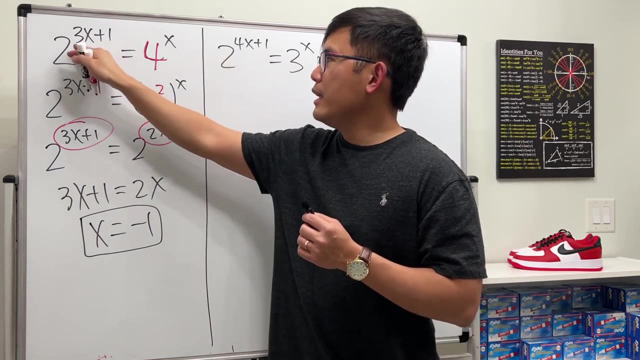 one being equal to two x and then solve this, move this to here, so we get x. x is just equal to negative one. that will give us negative two. that will also give us negative two, and it's always a good habit. plug back in, you will get four to the negative one, which is one over four, and you get. 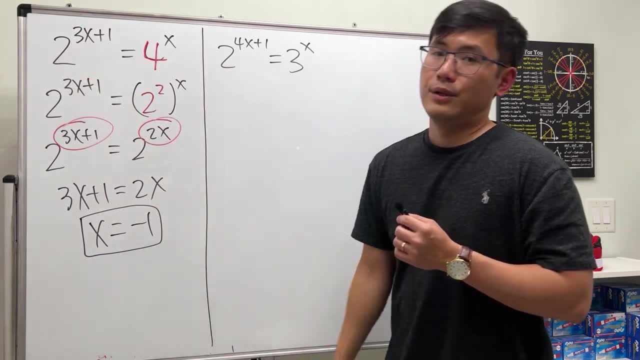 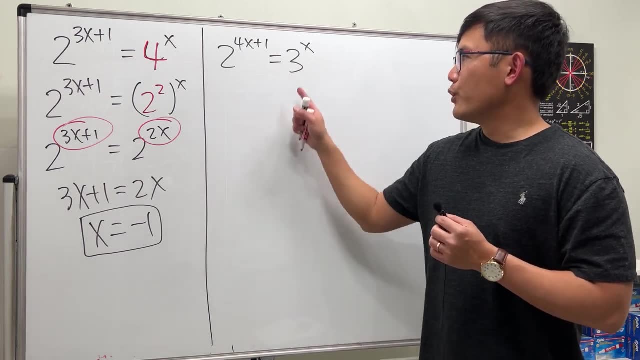 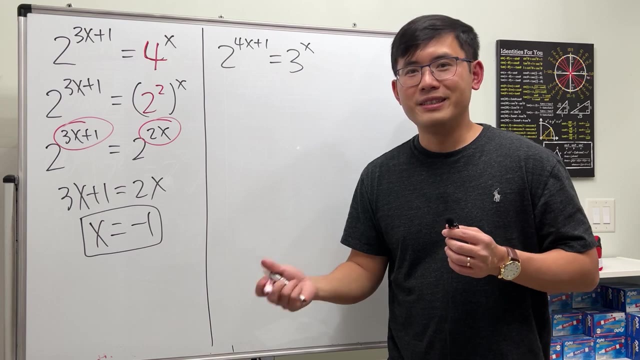 negative two right here. altogether two to a negative two. you get one over four. so x equals negative 1. done now for this. unfortunately, we cannot do that anymore. we cannot write 3 as a 2 to the 5th power. you could, why not? yeah, why not? i just remembered you. why not ready? 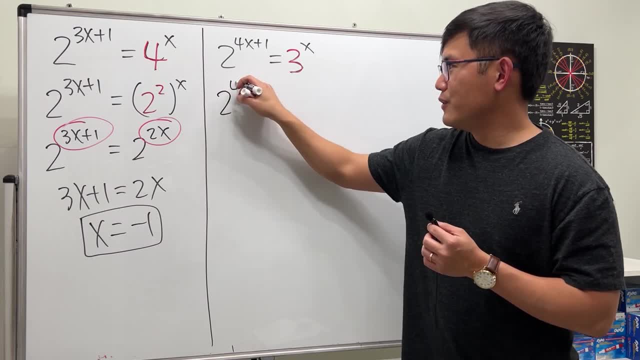 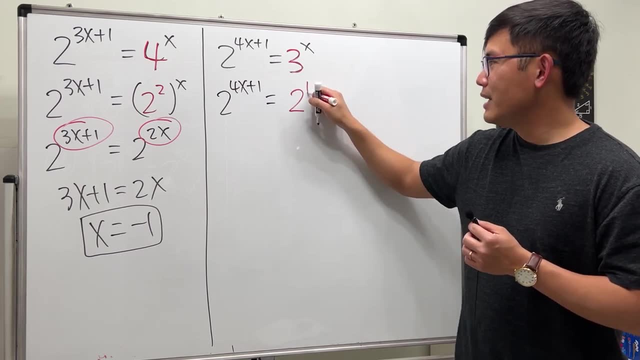 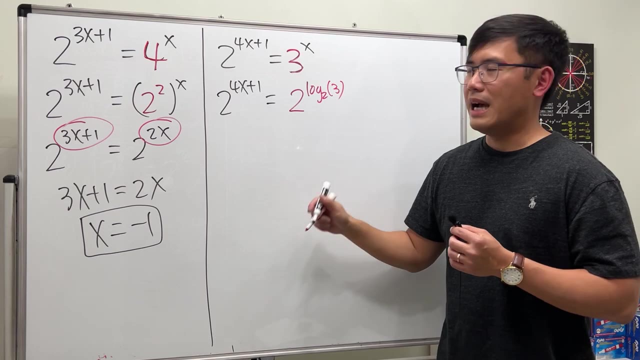 three on the left hand side, i'll keep it two to the four x plus one. but on the right hand side, ready, i'm gonna write three as two to the log base. two of three, oh, look this, and now we'll cancel. we'll still get a three back, and then we raise this to the x power. how's that? of course. 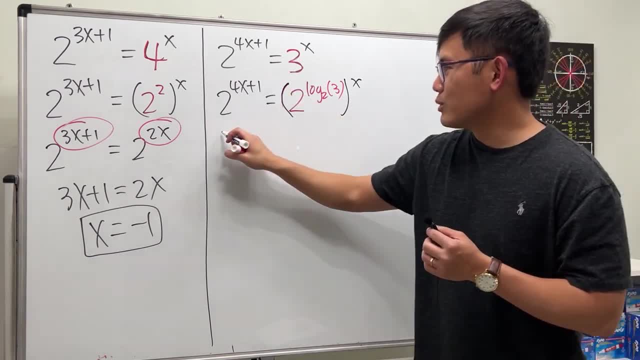 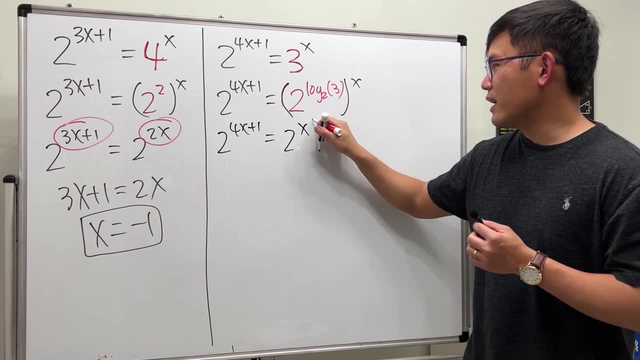 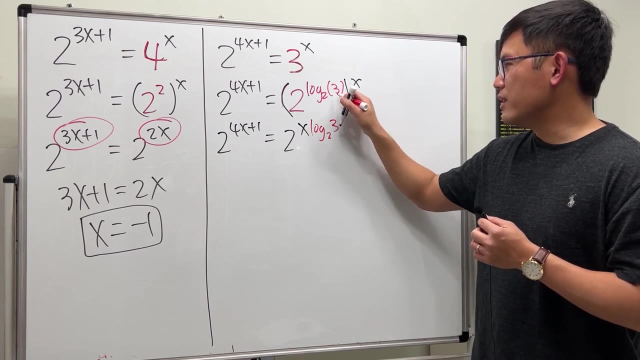 it's okay, yes, and then do the same thing. so we have two to the four. x plus one equals two, and then let's just multiply x, usually put at the front, because i don't want people to see that x is same, except for logs, not so. and you don't really need a parentheses because we only have a three. 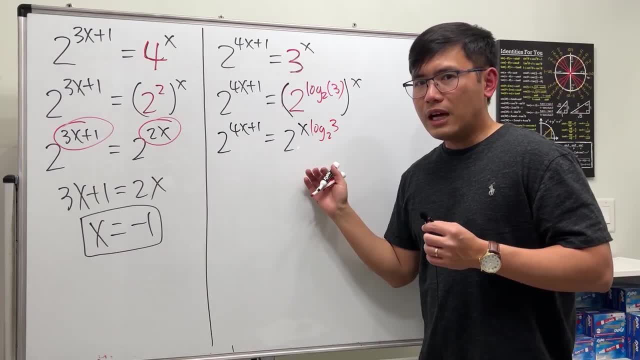 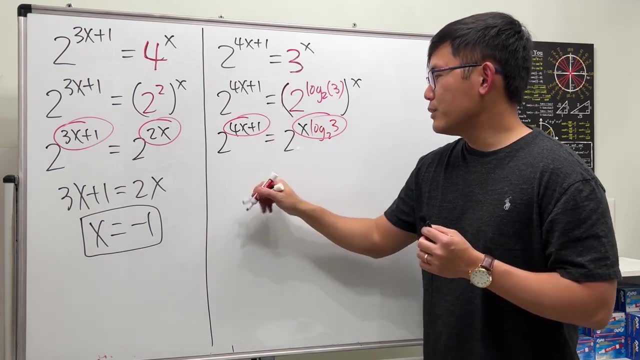 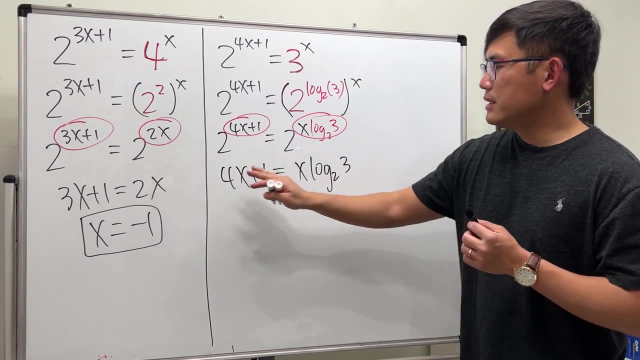 in inside of the log. so this is okay, so this is what we have. and then do the same thing. the exponents have to be equal, right, because the bases are the same now. so we are looking at: 4x plus 1 equals x times log base 2 of 3. move this there and move the 1 here, so we get 4x minus x log base 2. 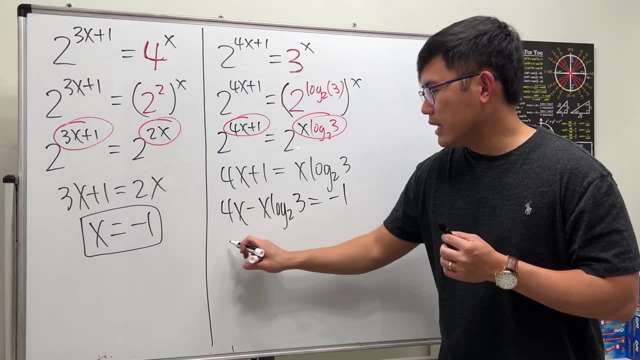 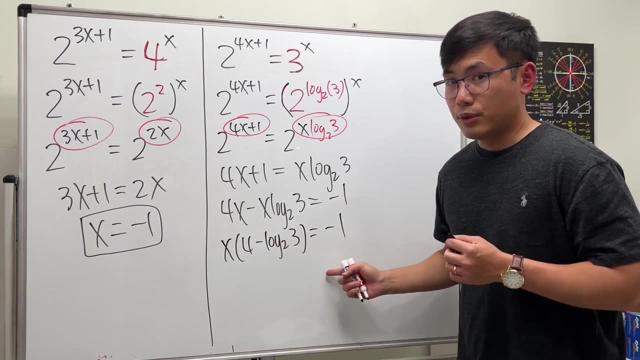 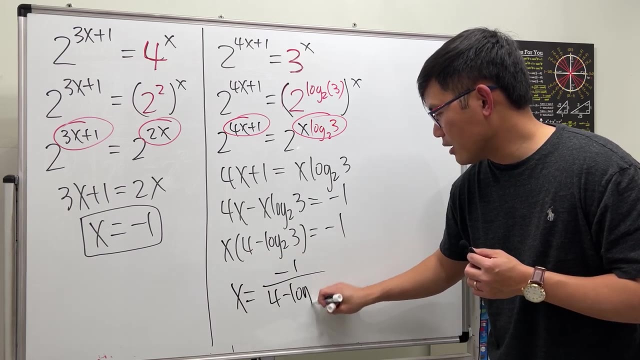 of 3 equals negative 1.. factor out the x and then 4 minus log base 2 of 3, this is equal to negative 1, and then just divide down both sides. so x equals negative 1 over 4 minus log base 2 of 3.